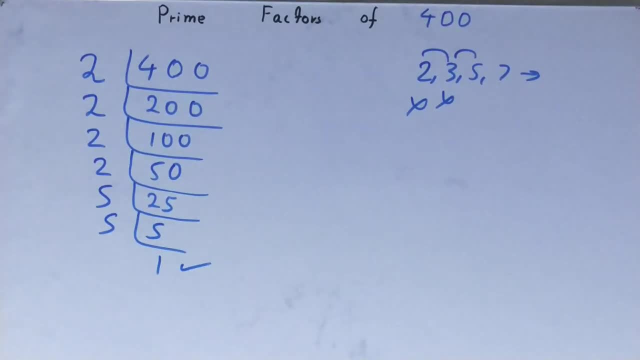 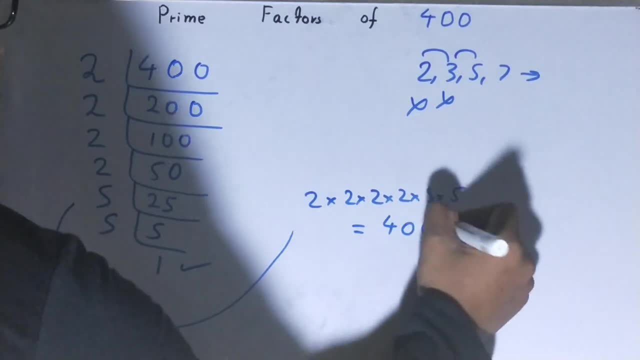 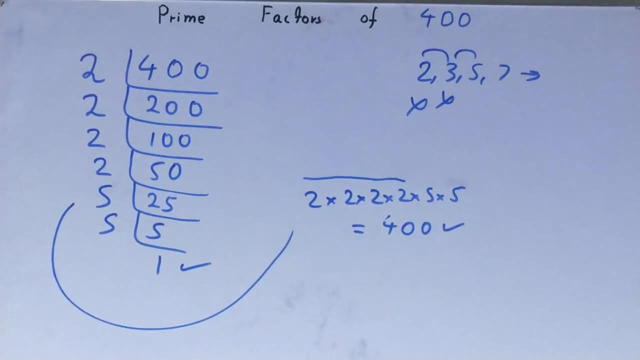 right or not, you can multiply them, and if on multiplying you have the number back again, that means your calculation is correct. if not, you need to recheck. you can also write it in a different way. you have four times two, so you can write it as two raised to power four, you have two. 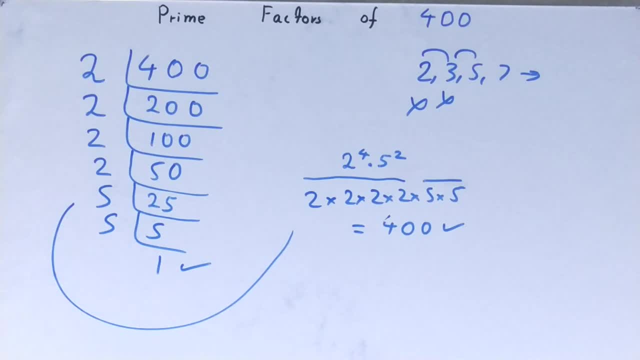 times five, so you can write it as five raised to power two. okay, so you can write it this way or this way, it's up to you. so this was all about practice. prime factors of 400. so if you like the video, please do the like button. do consider subscribing. and thanks for watching. 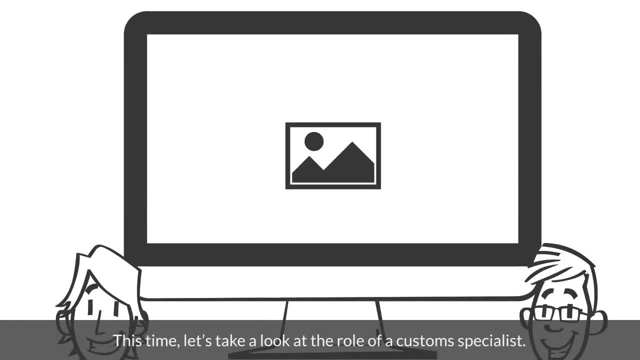 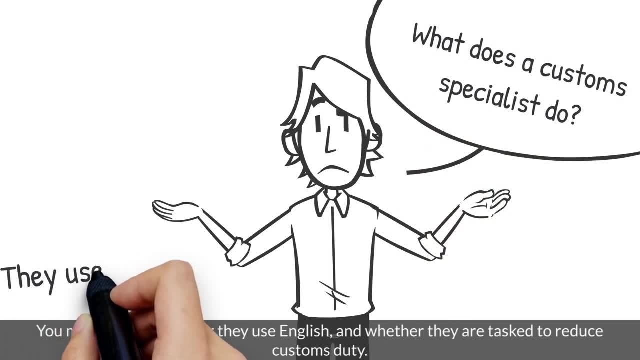 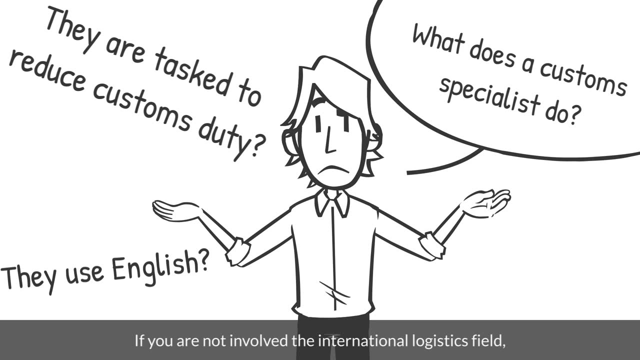 This time, let's take a look at the role of a custom specialist. What does a custom specialist do? You may wonder whether they use English and whether they are tasked to reduce customs duty. If you are not involved the international logistics field, you may not be familiar with the role of the custom specialist and you 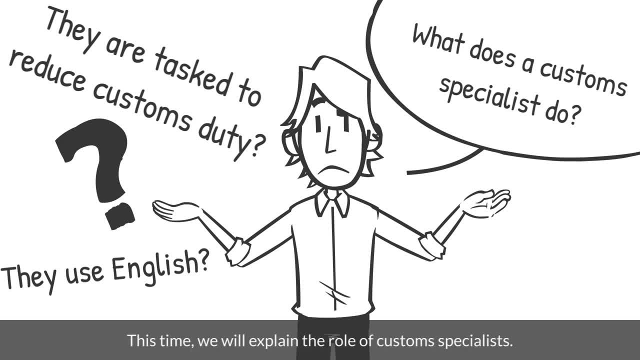 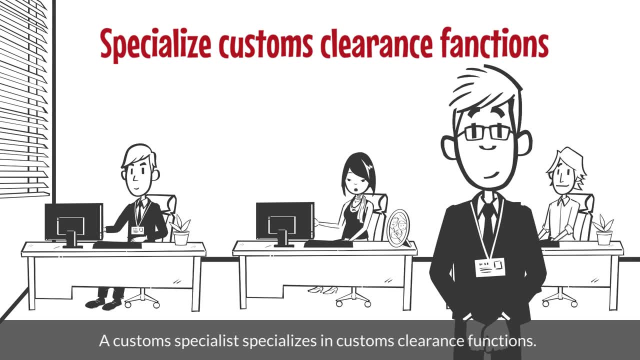 may not be able to understand the role. This time we will explain the role of custom specialists. A custom specialist specializes in customs clearance functions. They will receive a job request from another company- shipper and consignee and submit the documentation to receive an approval when importing. 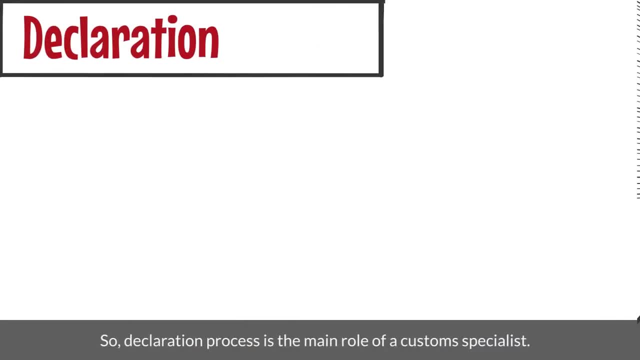 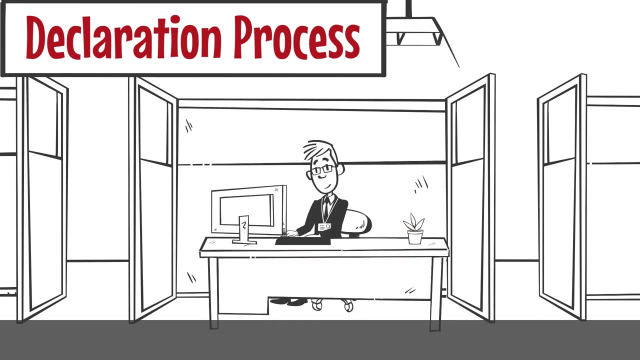 and exporting cargo. So declaration process is the main role of a custom specialist. We will explain what they do and how they work in detail. When a custom specialist receives a job request from another company, they will submit documentation to the customs office. They will receive.